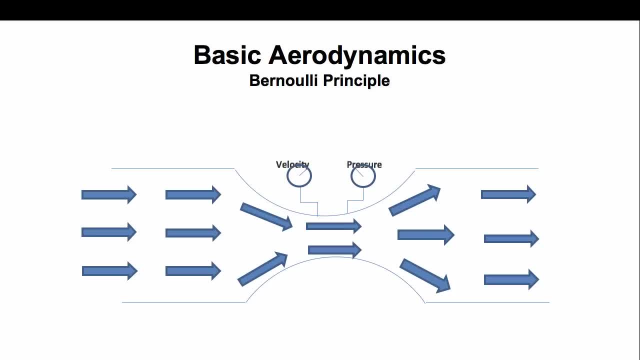 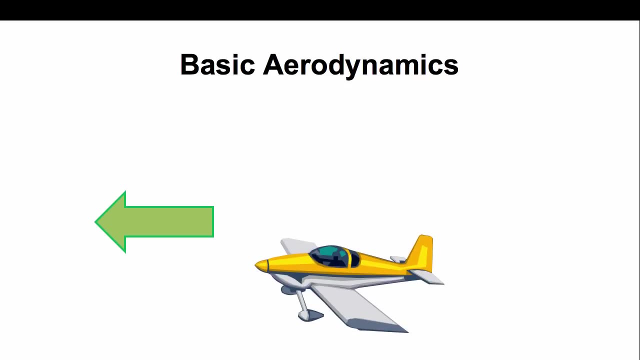 that every time the velocity increased or decreased, the pressure would have the opposite effect. In this slide we will define a very important force that would help us understand the future concepts. That force is the relative wind. The relative wind is simply the airflow that. 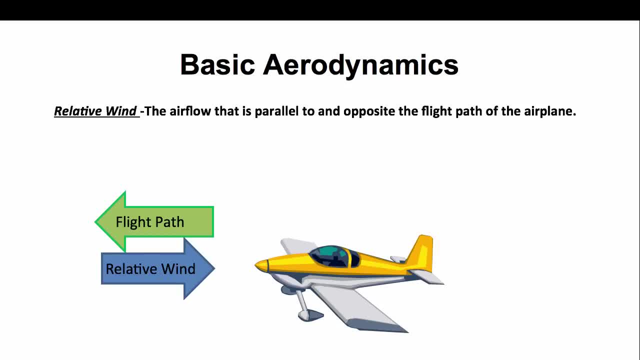 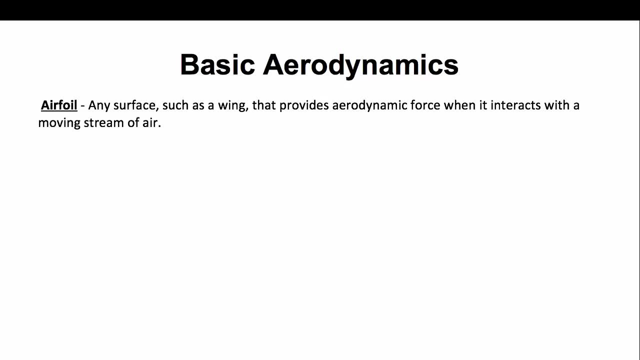 is parallel and opposite to the flight path on the plane. The relative wind is when the the airplane, An airfoil, is any surface such as a wing, that provides aerodynamic force when it interacts with a moving stream of air. When given a flight path and an opposite relative wind, it's important to remember that the 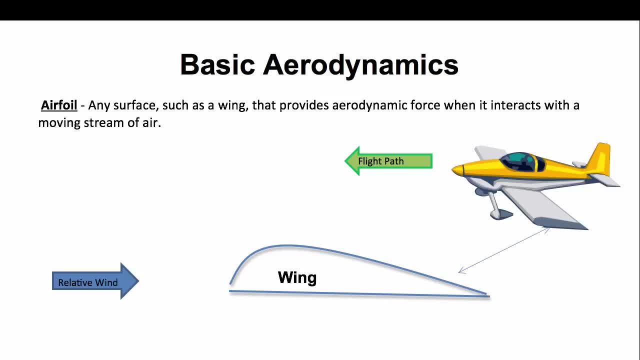 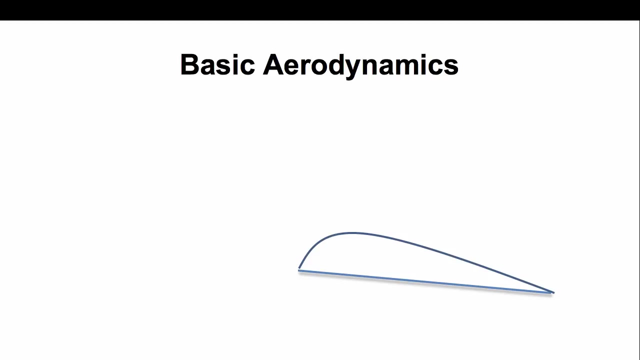 airflow over the surface of the wing will have a higher velocity than the airflow under the wing. It's also important to note that the circulation of the airstream about the airflow is an important factor in the generation of lift, The camber. It is the characteristic curve of the airfoil's upper and lower surfaces. The 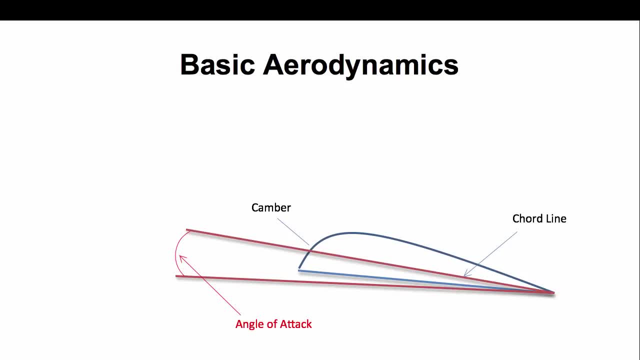 chord line is an imaginary straight line drawn through the airfoil and the direction of the relative wind. The chord line is a very important determinant of what's called the angle of attack. The angle of attack is a function of the airfoil's surface, and so is the airfoil's flow. 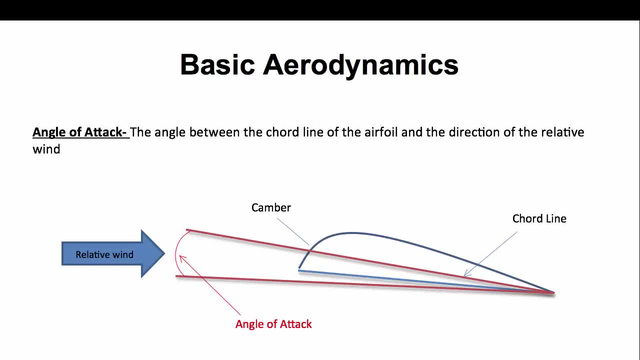 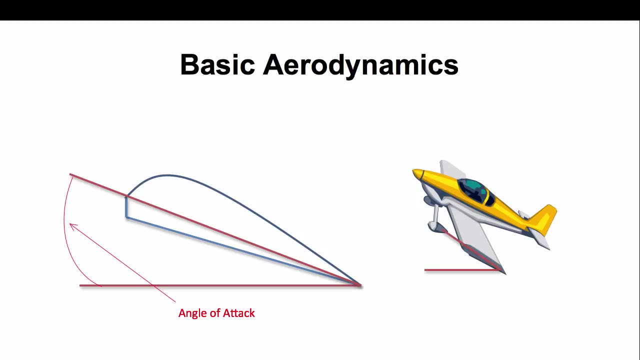 attack is simply the angle between the chord line and the airfoil at the direction of the relative wind. in this slide we will learn that as the angle of attack increases, the lift also increases. please note that the lift acts perpendicular to the relative wind, regardless of the angle. 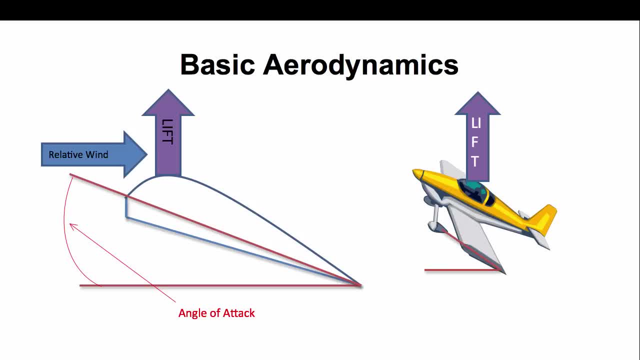 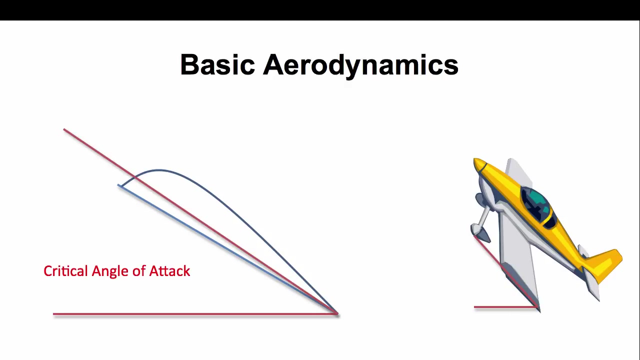 of attack. according to Bernoulli's theorem, the increased speed of the air on top of an airfoil produces a pressure drop. this lowered pressure is one component of a total lift. however, when the angle of attack is increased beyond the maximum allowed, the lift is decreased. 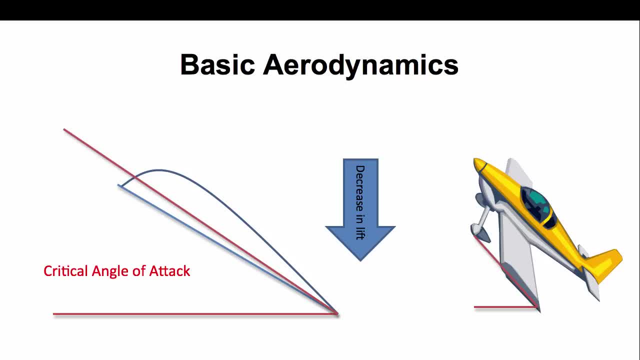 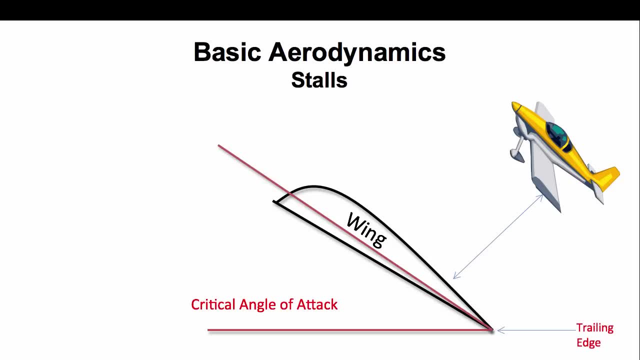 this causes what's called a stall. as we mentioned earlier, a stall is a result of a critical angle of attack. it is also caused by by the disruption of the air flow from the upper surface of the wing or airfoil. The air flow then separates at what's called the trailing edge. 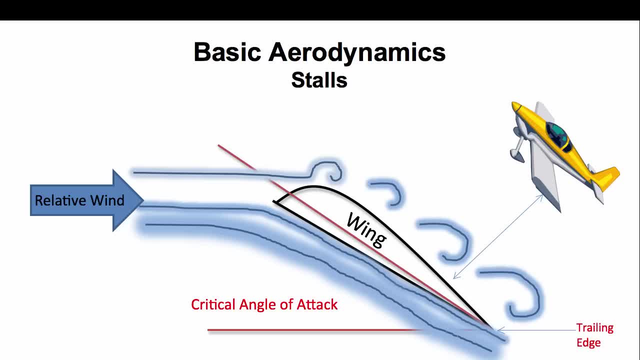 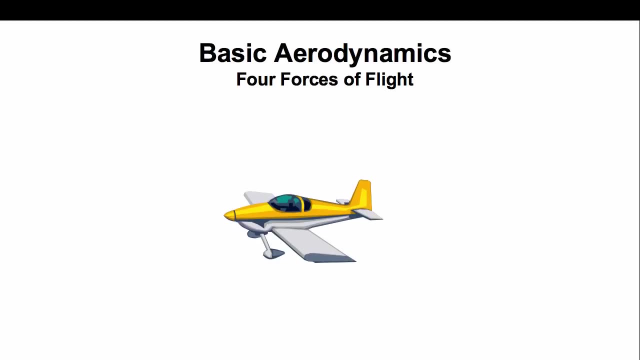 The air flow progresses forward until the wing is fully stalled. Therefore, a stall is a rapid decrease of lift caused by separation of air flow. In this slide, we will learn about the four very important forces of flight. The challenge to understand what makes an airplane fly starts with learning the four. 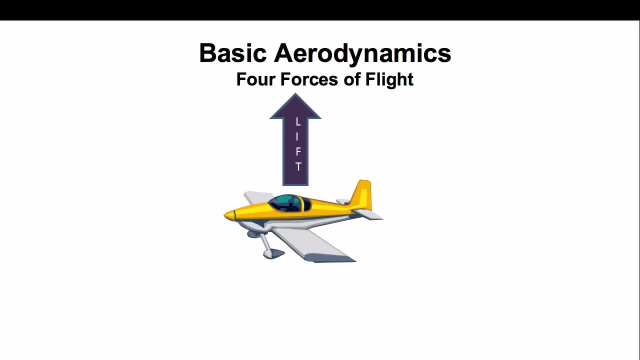 forces of flight. During a flight, the four forces of flight, The four forces acting on the airplane, are: lift, weight, thrust and drag. Lift, as we discussed earlier, is created by the effect of air flow over and under the wing. The weight of the airplane, that is, the force caused by gravity. 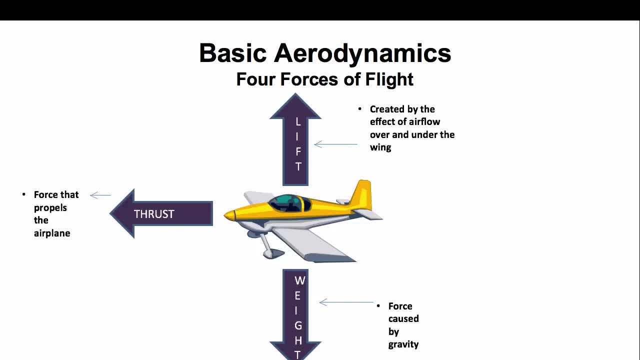 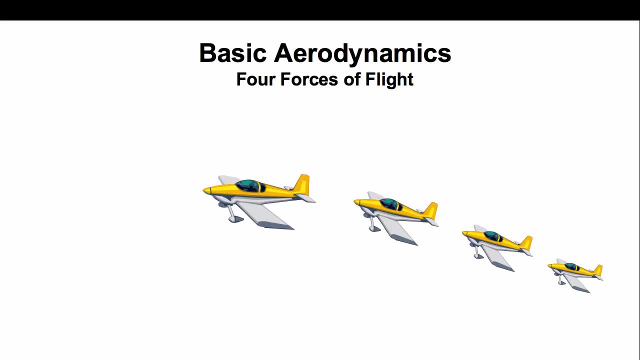 The thrust, that is the force that propels the airplane. The thrust, that is the force that propels the airplane. And, finally, the drag, which is the force that limits the speed of the aircraft. The drag, which is the force that propels the aircraft.